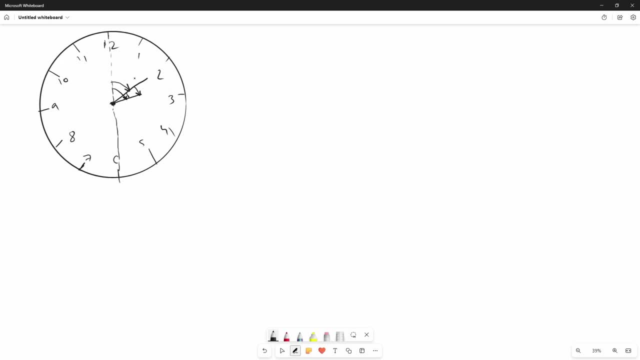 From minute to hour hand. So we will use this assumption in our calculation. So suppose the time and the other. by the way, other assumption that we will take is that our time is in 12 hour format, So let our time be some h hours and m minutes. 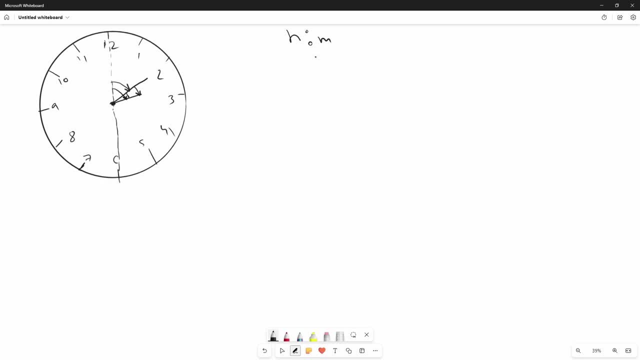 am pm, doesn't matter. So since we know that the minute hand covers 3.7 full circle in 60 minutes, 60 minutes is covered in 360 degree by the minute hand. So that means one minute is covered in 360 by 60. That is six degrees. 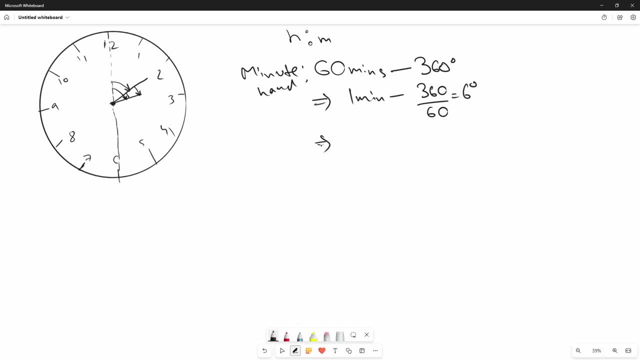 So therefore, minutes in M minutes, the angle covered by the minute hand will be 6, 6 M- sorry in, not H M degrees. that's the first value. so what we have found, that a 6 M is the angle covered by the minute hands from the reference and in clockwise. 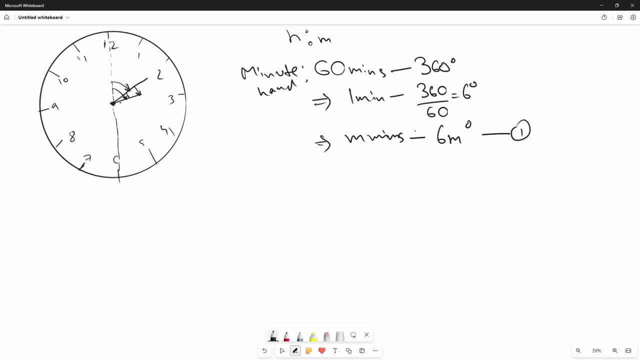 direction reference hand is nothing but an imaginary. we have to take in references that the this direction is can be considered. the next is the our hand, our. so, as we know, in 12 hours the our end completes one revolution. that is 360 degree. but we can't just write 12 hours, 360 degrees. we need to understand. 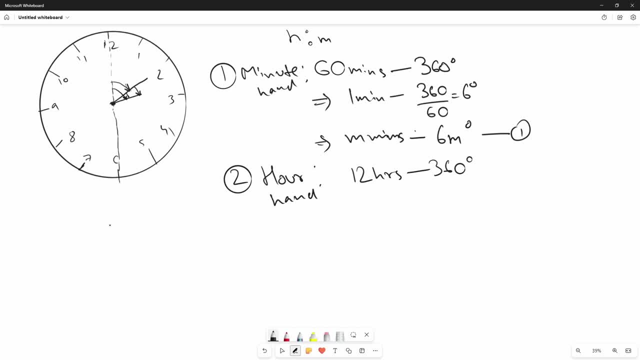 that when, as long as suppose, we have to walk now, where the minute hands is at 12 and our hand is at 2, so that's fine, but as the minute hand passes with time, the hour and also ships, so the, the Sophie can't take, we can't just take the angle between. 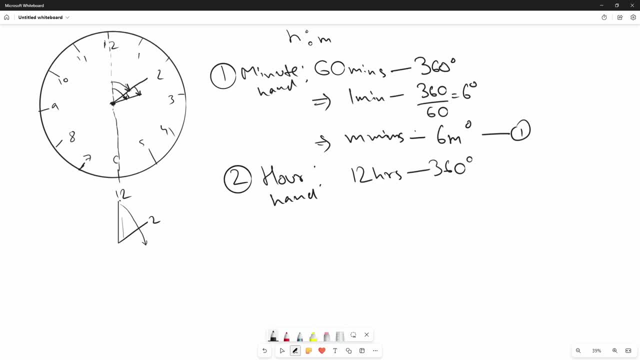 the reference and to. instead we have to take the angle between the reference and the our-hand move slightly after 2. so because of that, first we will convert this to minutes. that is, 720 minutes is taken by the our hand to complete 360 degrees. so 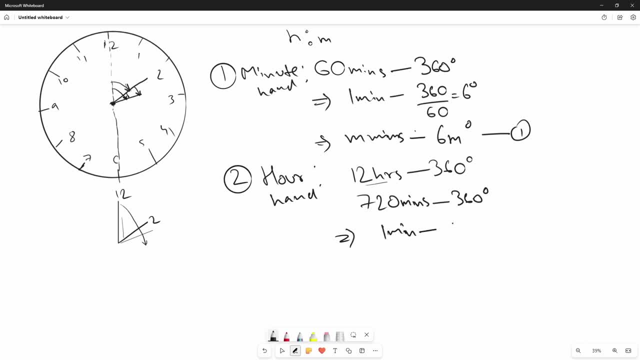 therefore, in one minute, our hand takes half degrees and therefore so, since its HR's and n minutes have passed, so we'll have to take. the total time that has passed is 60 H, 60 H plus M. right, I have fully converted it to into minutes one. 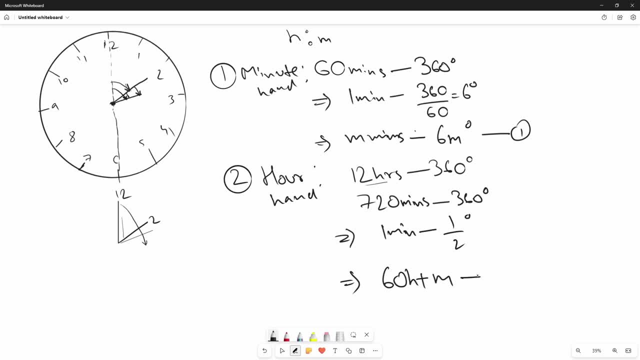 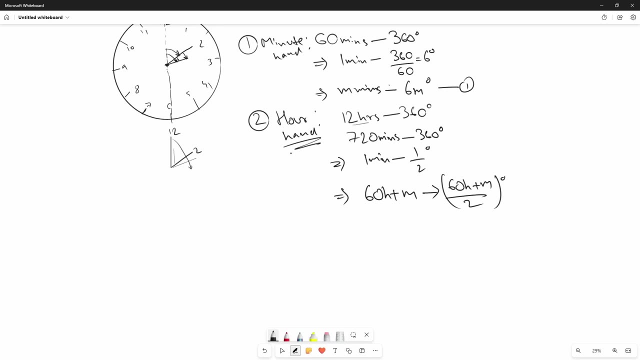 hour is 60 minutes of 60 H, then then M minutes, so that will give 60 H plus M by 2 degrees for the hour. so all that is left is to calculate the angle between the hands, which is angle formed by our hand minus angle formed by minute hand, so which is equals to 60 h plus M by 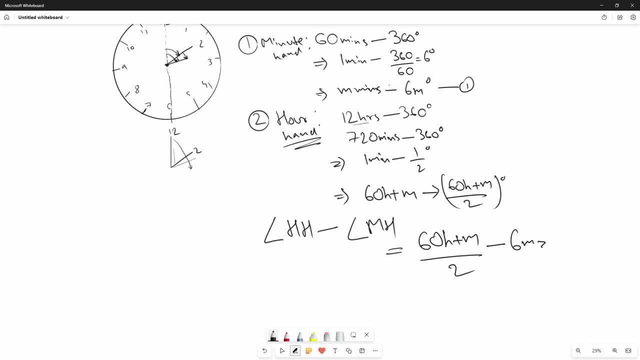 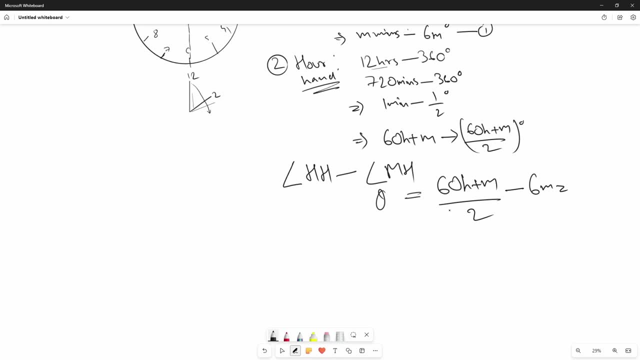 2 minus 6 M and that. so if I, if we keep our angle as the theta, then our theta will be the angle of 60 H plus M, which is 60 H plus M minus 60 H plus M, that is will be 60h minus 11 minute by 2. so we have found how to find the angle between the hands. 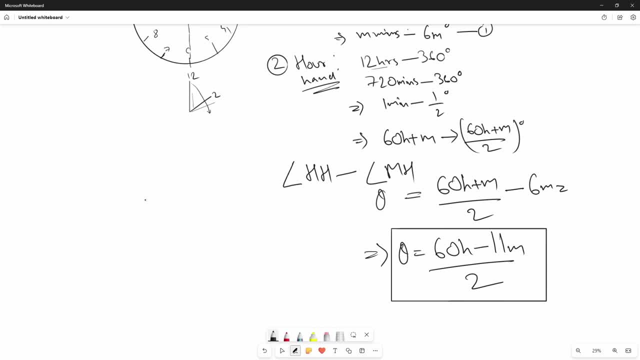 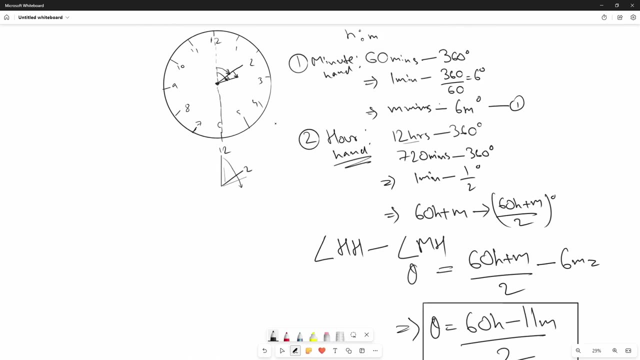 so there are two things we need to make sure of. suppose, if we input our hours and minutes into the formula, sometimes it can happen that our theta comes as a negative value, which is because that in our assumption we have assumed that the hour hand in clockwise direction. 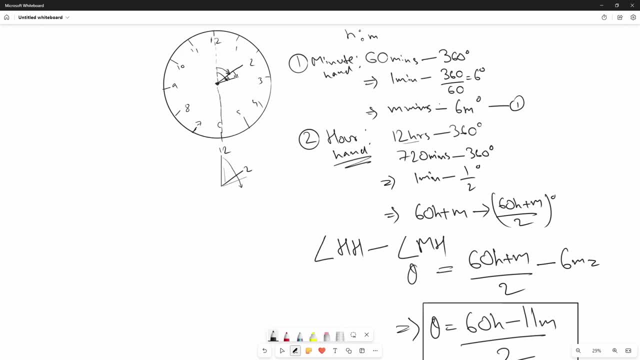 the hour hand lies after the minute hand, but sometimes it can be possible that the minute hand can come after the hour hand. suppose in the example of let the time is 7.45, so 7.45 will be somewhere, the hour hand will be 7 and 8 and the minute hand will be at. 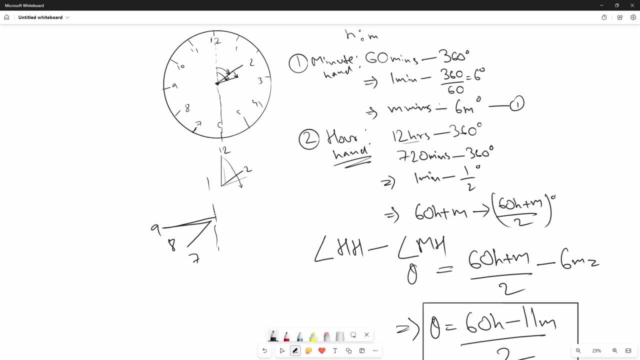 9.. So, as you can see that, with the reference the hour, the minute hand comes after the minute hand comes after the hour hand. so this, a possibility is also there, in which case we have to take the positive value. so if this, if theta is comes less than zero, take the positive value, take the positive. 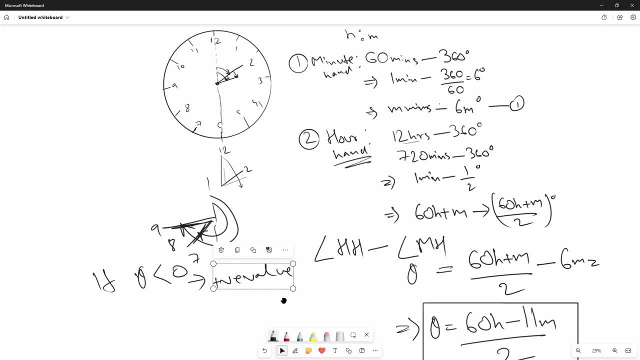 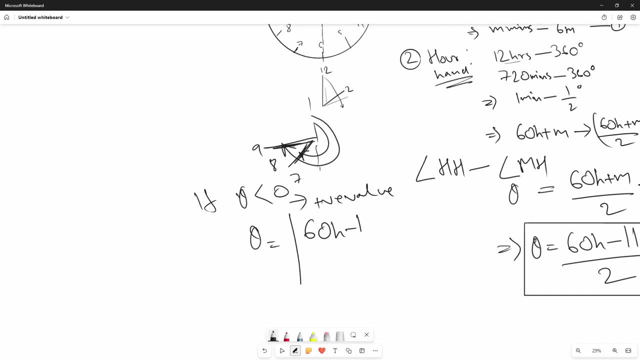 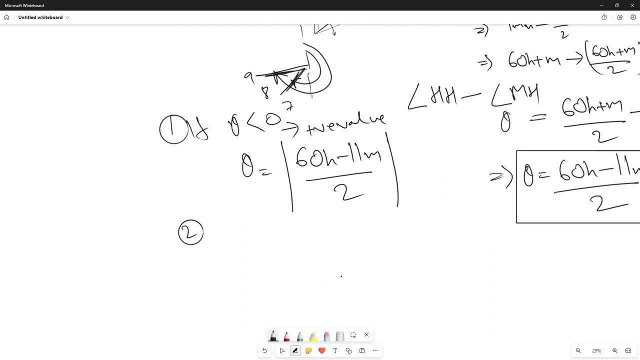 value. so because of which we can generalize This as theta is equals to mod of 60 h minus 11 m by 2, where mod gives the positive value. this is the first consideration. the second consideration is: it is possible. it is possible that the angle can come more than 180 degrees, for example. let's say, let's say 10 o'clock. 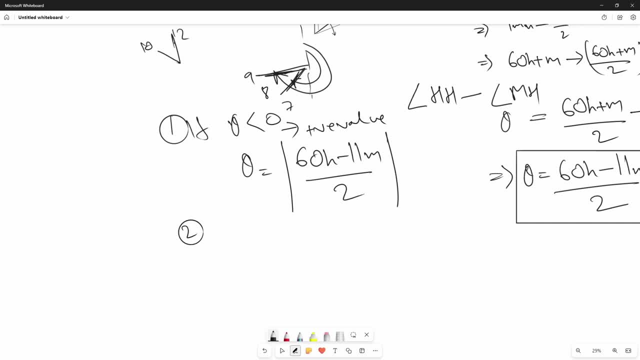 10 o'clock, Yeah, So see the 10 o'clock: 10 o'clock, Yeah, So for 10 o'clock the minute hand coincides with the reference. if we take the direction, then you can see that the angle will be calculated between hour and minute hand in the clockwise. 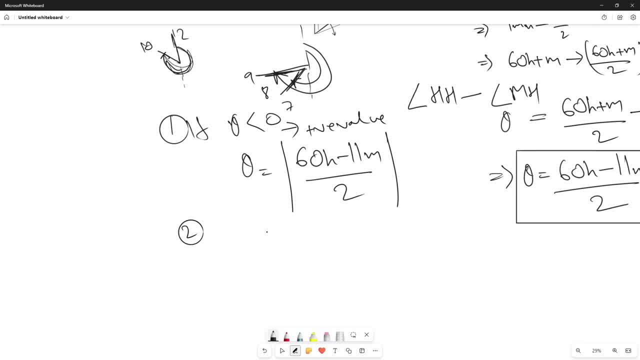 direction, which is this angle. so you know, if, if, if theta comes more than 180 degree, then you need to subtract it from 360.. Yeah, Yeah, Yeah. So theta becomes 360 minus 60 h minus 11 m by 2. if theta becomes one more than 180, then 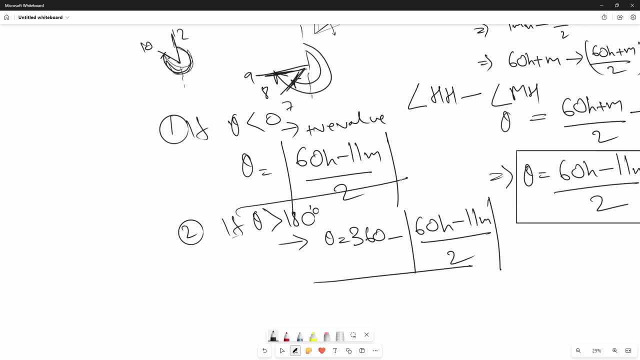 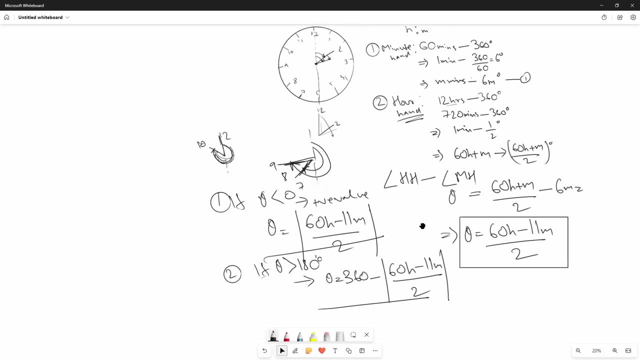 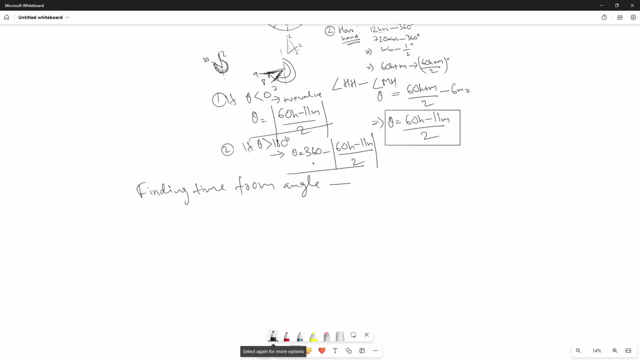 you apply this formula, otherwise, apply this formula. So this is how we calculate the angle between the hour and the minute hand. now one, since we have found out How to find angle difference from the time, the converse is also true, that is, finding time from angle. how we will do that is that depends on two cases. one is when minute hand comes. 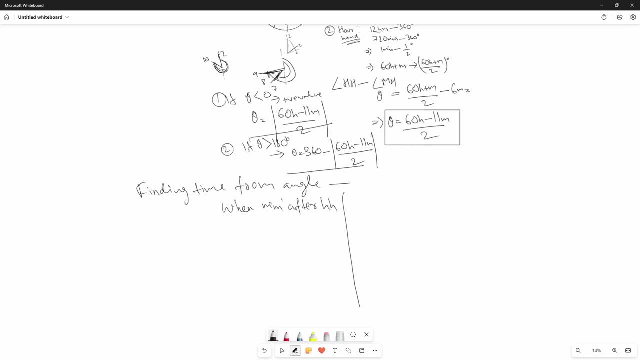 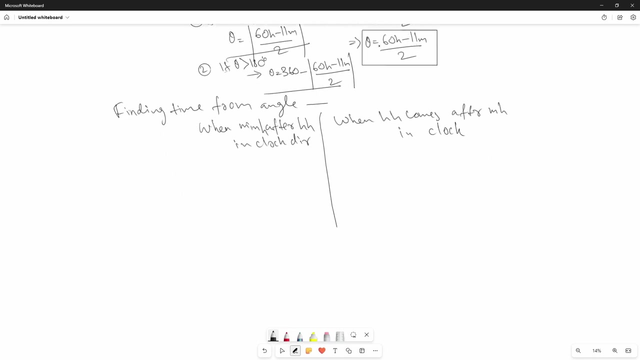 after hour hand. minute hand comes after hour hand in clockwise direction. and the second is when Our hand comes after minute hand in clockwise direction. okay, So our formula for theta is 60 h minus 11 m by 2, so when minute hand comes after hour. 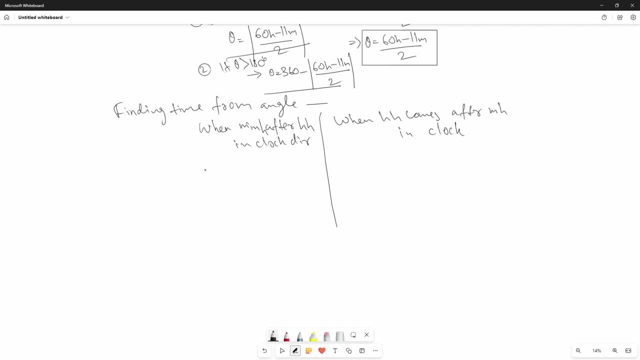 hand, the angle goes negative, because of which we have to take minus theta to break the mod over here. to break the mod over here. Yeah, So it becomes 60 h minus 11 m by 2, or m is equals to 60 h plus 2 theta by 11, why I have 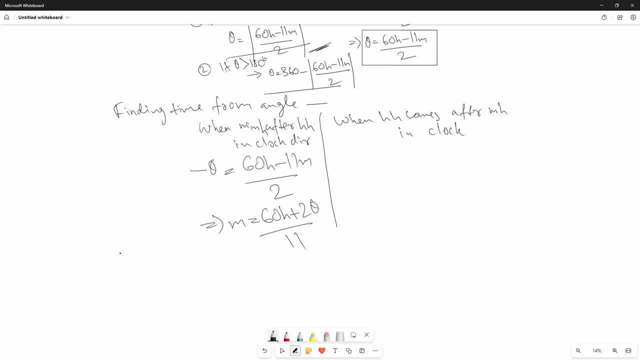 made m as the subject of formula, because h can be any value between 1 and 12. because of the hour hand, it is the minute that we need to be focusable. similarly, when hour hand comes after minute hand in clock, The theta will be positive. so we break the mod. 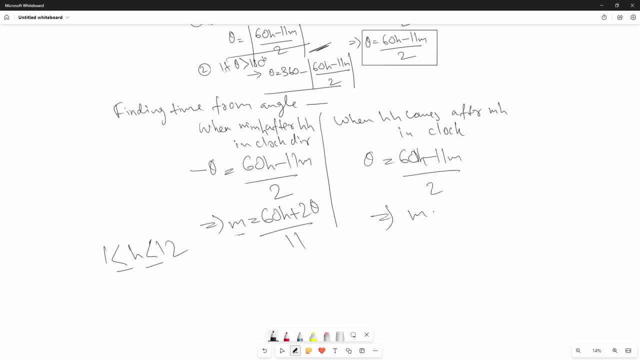 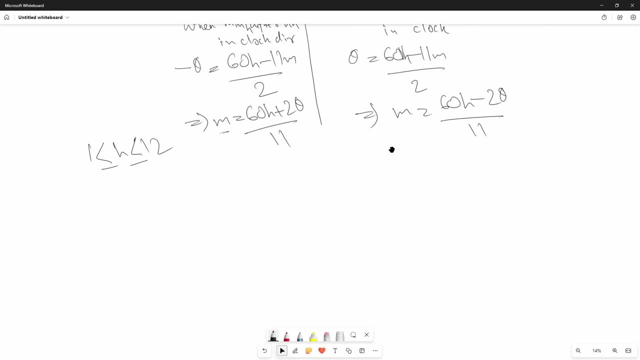 Minus 11 m by 2, or m is equals to 60 h minus 2 theta by 11. okay, Now how to work with these two formulas. suppose we need to find time such that the angle difference is 45 degree. We take the hour hand as 1.2.. 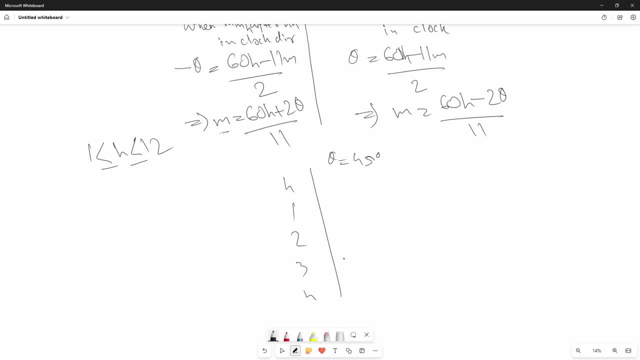 Yeah, 1.2, 3 and 4 for now, the for the remaining, that is, 5 to 12, you can work it out. So first part of the algorithm is: find 60 h. find 60 h. sorry, so this will be 60, 120,. 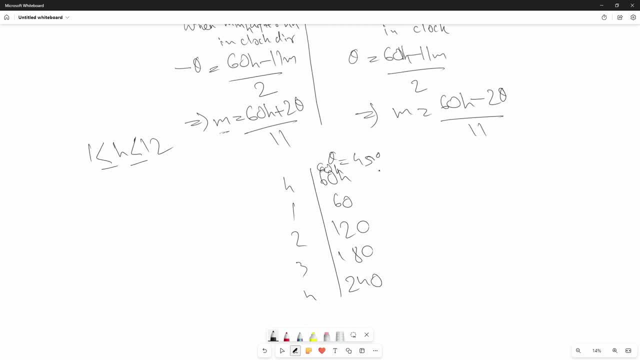 180 and 240.. The next part is find 2 theta, which will be 90 for all four. Okay, Third part of the algorithm is we need to check if 60 h is less than or greater than equal to 2 theta. 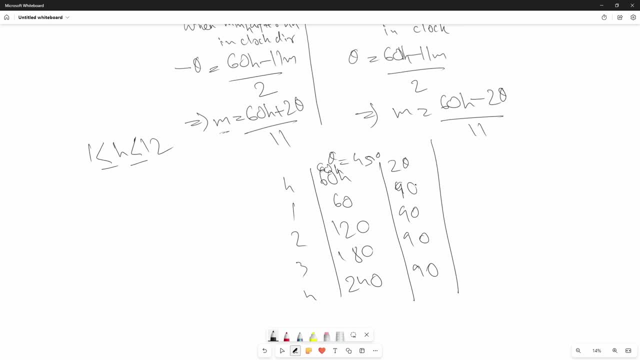 If 60 h is less than 2 theta, which is the case for when hour hand is at 1, hour is 1 in the time format, h and m, h, hours and minutes Anyway. So if 60 h part is less than 2 theta, 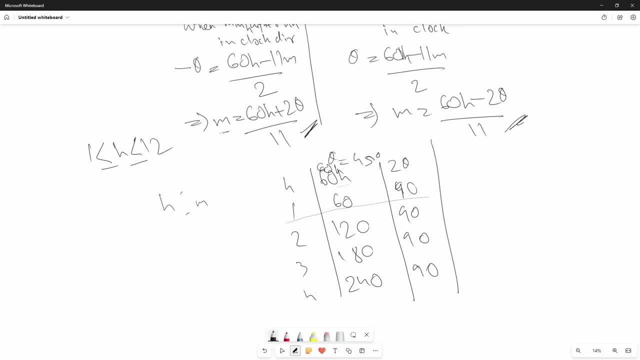 We need to apply this formula, otherwise this formula, that's the part, that's the whole algorithm. So we need to. for first case, we need to apply the first formula, which is 60 plus 90 by 11, which is equals to 150 by 11.. 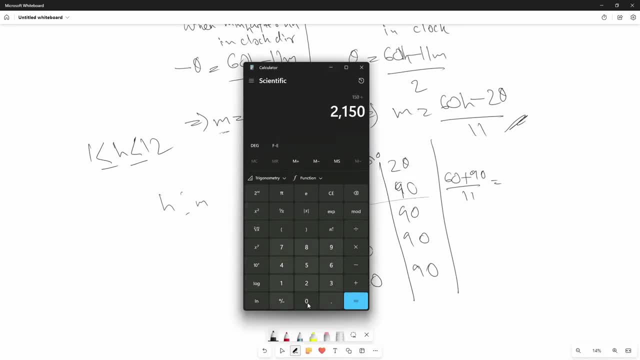 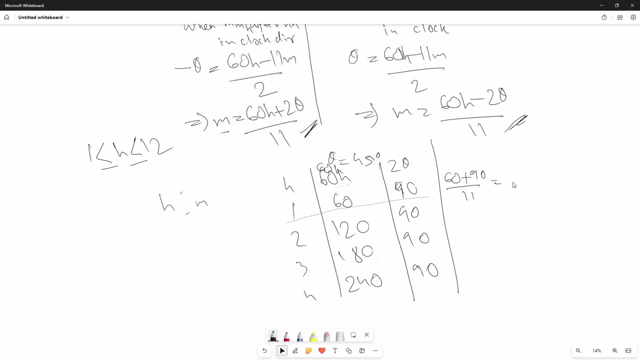 If I take my calculator, Okay Okay, Okay The first time, So no 153.. It will be somewhat around 13 minutes and point six three minutes. So this will be 13 minutes and point six three is almost around 36 seconds. 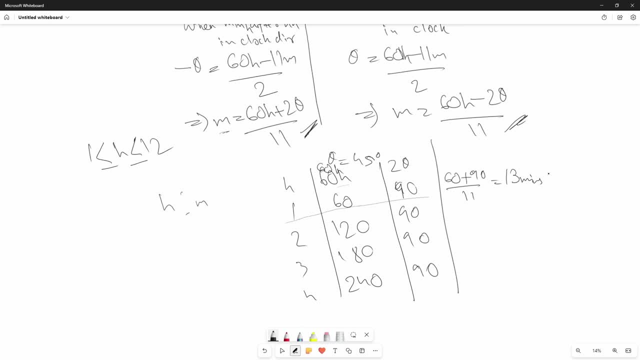 So we have For. so For Our first time we have found out that is one minute 3030 minutes, which is about half of the time. So it is basically one minute 30.. So that means this is the whole program minute. I mean one hour 13 minutes and 36 seconds. am, pm, doesn't matter once. 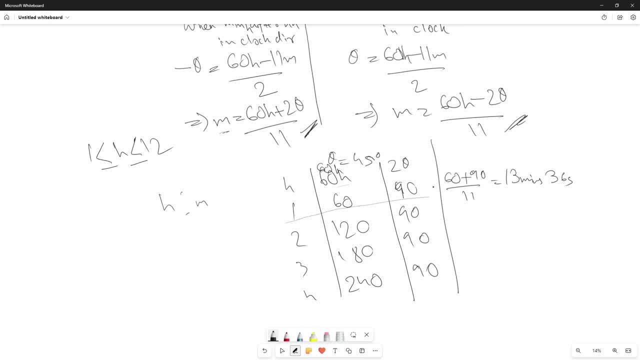 again in the second part we have, we will. for the second one, we will apply the second formula. since 60 H is greater than 2, theta, which is 120 minus 90, which is 30 by 11, which is equals to 2, 2 minutes 7, and this will be somewhat. 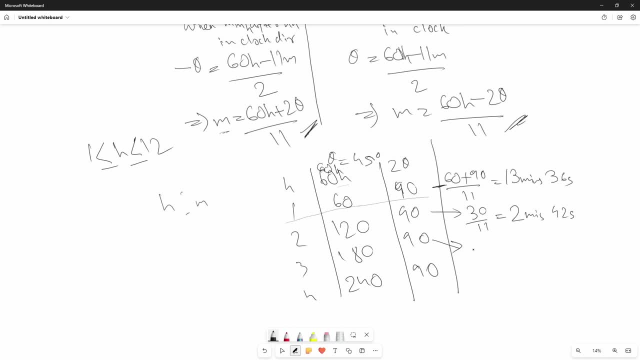 around 42 seconds. for third, it will be 90 by 11 because, once again, the second equation will be applied. this will be 8 minutes and one nine, two 12 seconds, somewhat alone. for the fourth one, again the second equation will be applied because 60 H is greater than 2 theta, which will be 150 by 11. 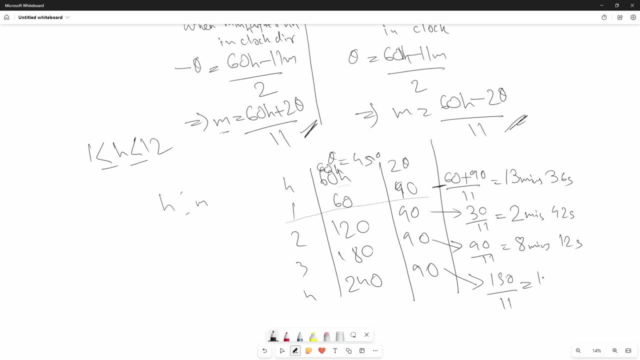 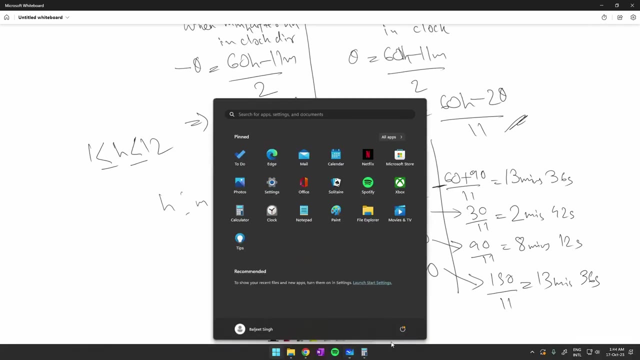 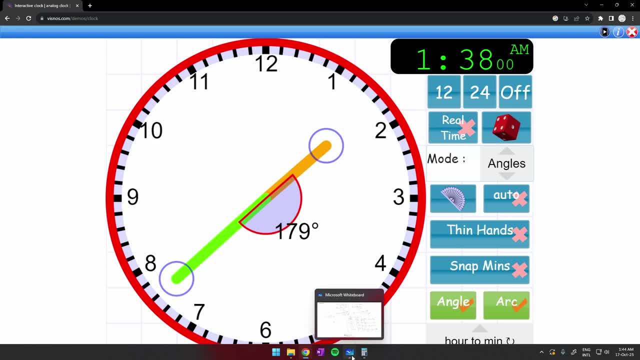 as well as the angles. so first we will test for a 1 hour 13 minutes and 36 seconds, the first. if we adjust this, you can see 36. okay, anyways, i'll stop at 37, if it's okay, 36. so, as you can see, our calculation is.